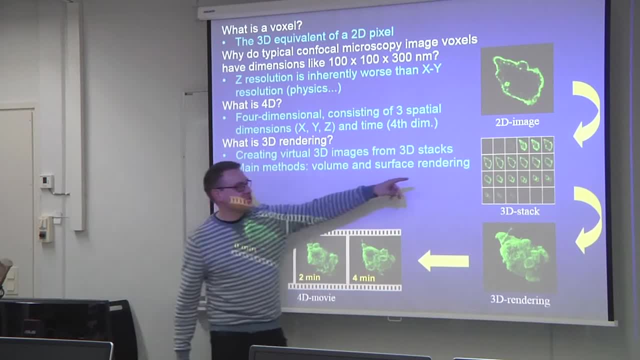 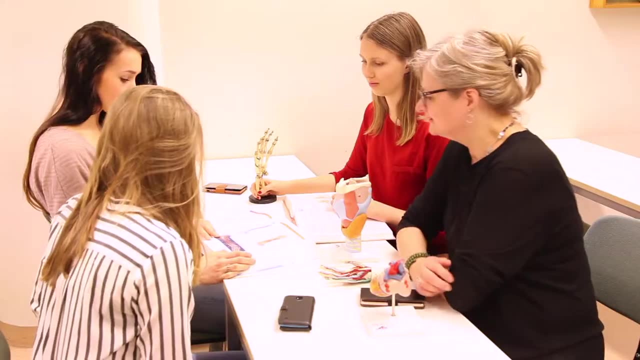 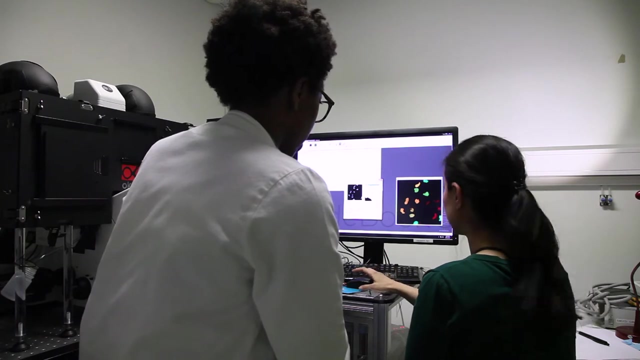 In BIMAI, students learn the theory behind many diverse imaging technologies. They learn the methodology and they learn how to apply them. in biosciences, The major subjects focus around imaging and they cover microscopy techniques, fluorescence methodology, physical basis of medical imaging. 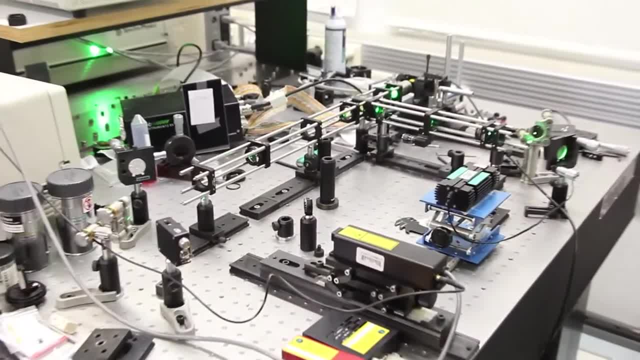 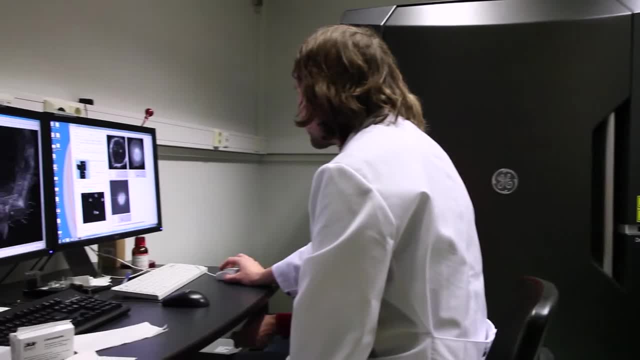 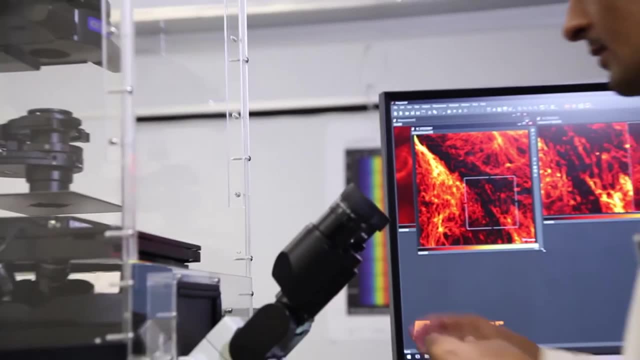 We also have nanoscopic imaging, biomedical instrumentation and digital image processing. Since biomedical imaging is strongly linked to technology and you learn by doing, we do offer practical hands-on and work demos in several of our courses, For example, in the microscopy classes. students have hands-on sessions at the microscopes. 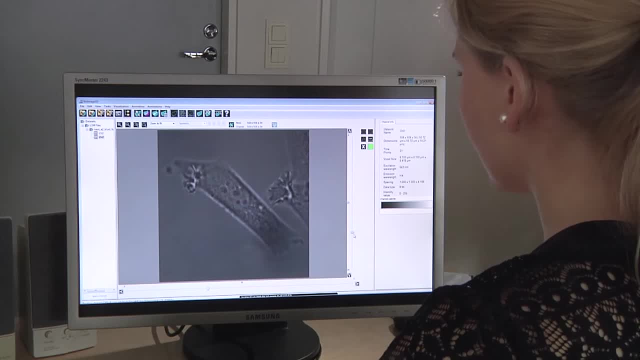 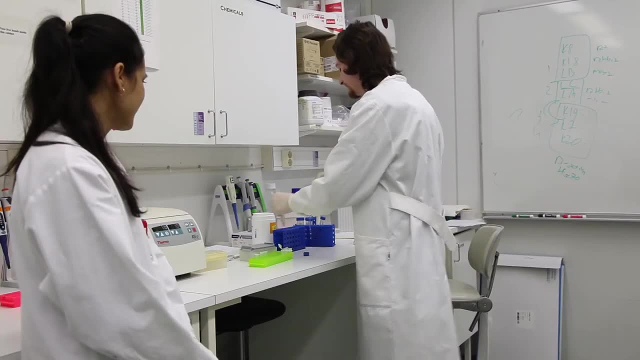 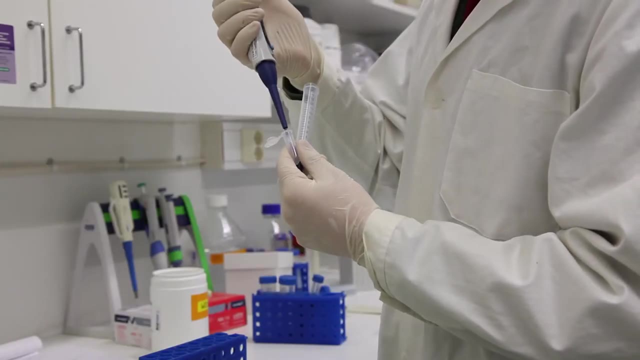 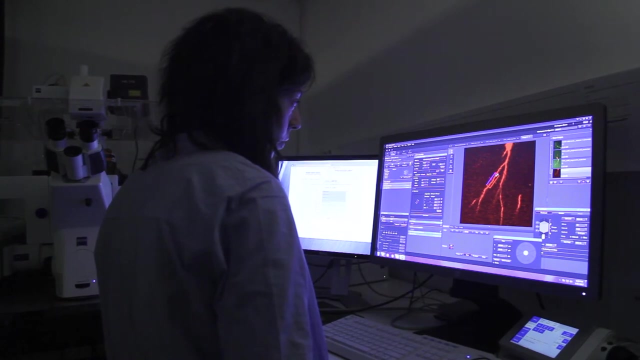 and also learn to do digital image analysis from examples from science. A very important aspect are the laboratory internship course and then the practical work for the master's thesis, where students choose to work in different research teams and to specialise in different technologies. Turku plays a central role in biomedical imaging in Europe. 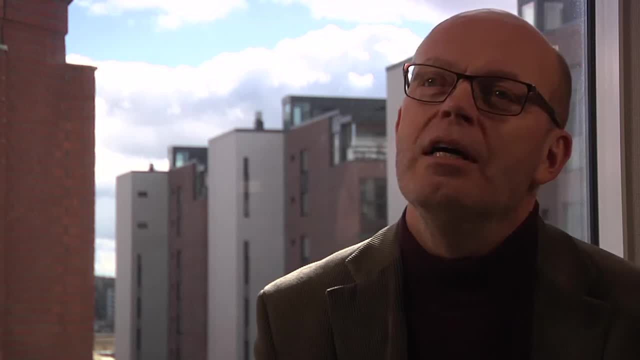 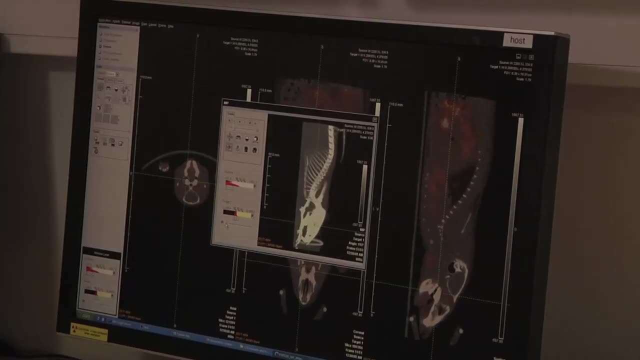 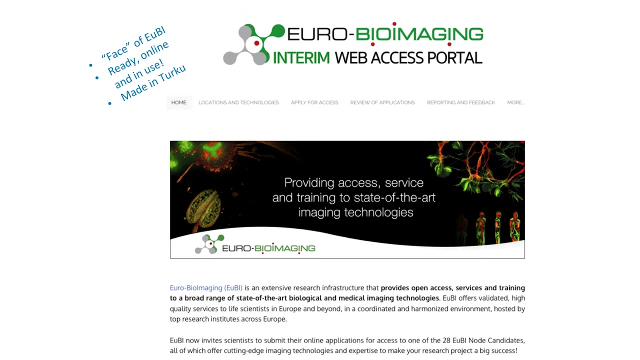 Turku PET Center is obviously the most visible part of our imaging facility. It is one of the largest research facilities in the whole world. Another key point is that we are not just a laboratory. we are now leading Eurobioimaging initiative and we are a key player in European bioimaging theme. 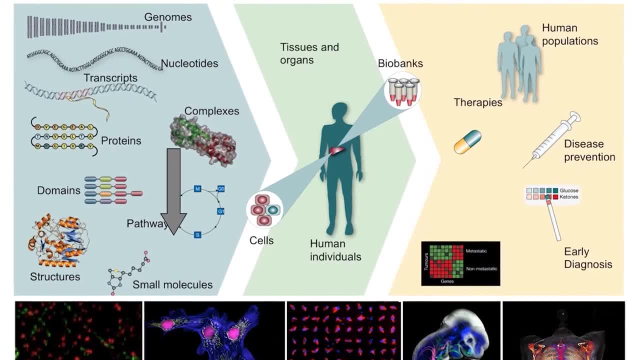 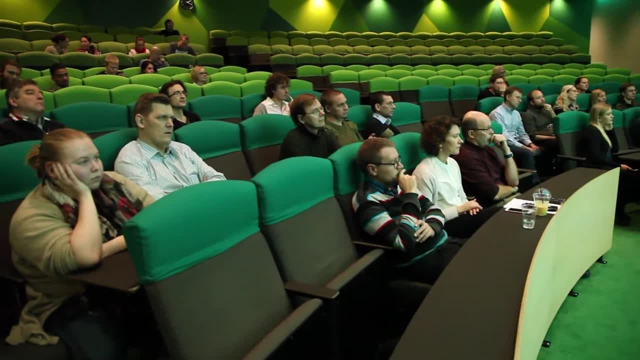 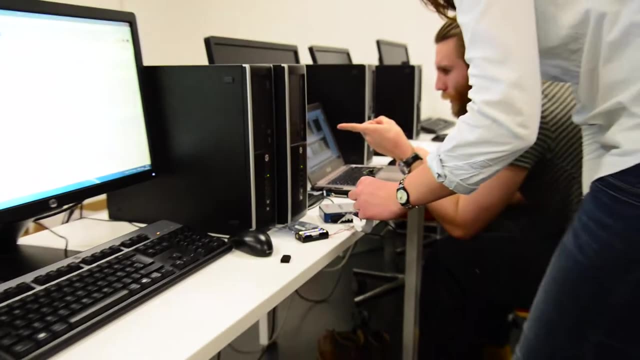 also at molecular and cellular imaging. So if you want to find what is best in Turku-East, then we have a seamless opportunity to image from molecules to men. BIMA as a program is multidisciplinary, so actually the team of students and teachers are all with different. 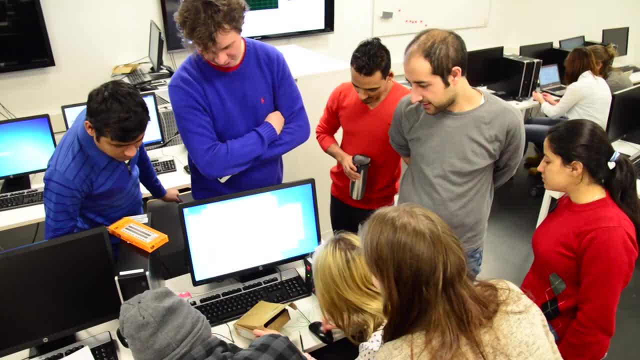 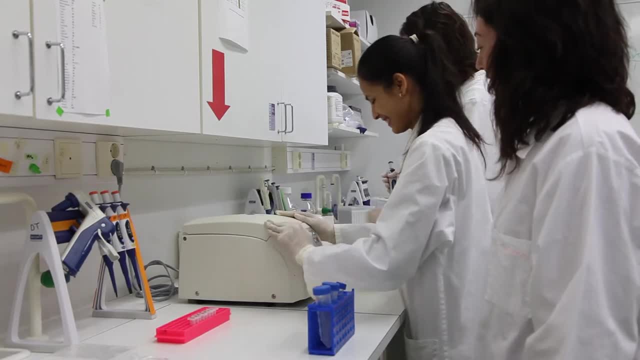 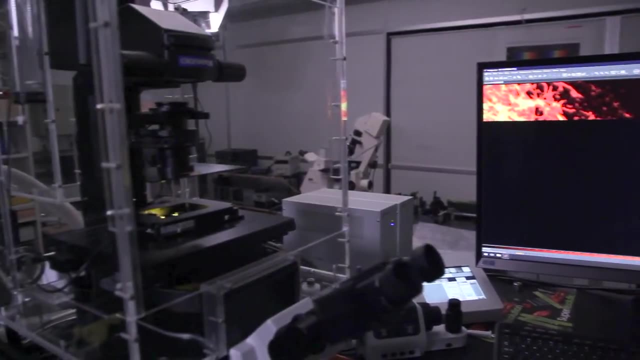 BIMA as a program is multidisciplinary, so actually the team of students and teachers are all with different backgrounds and it's a well-known fact that from crossing points of science, that's where all the innovation happens. If you're looking at the history of Turku, from development of instrumentation,